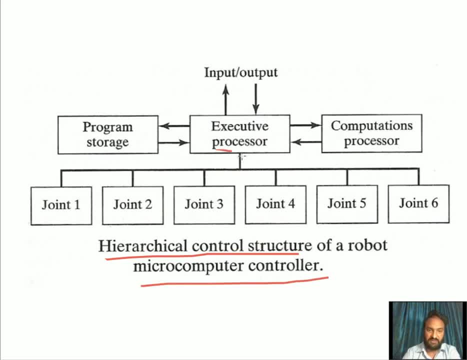 so joints are controlled by the, this one executive processor, we can say it as a robot controller. and then here is a program storage device that can be used your PC or personal computer, and then in robot controller, computation processors are there. how much degree it has to move. 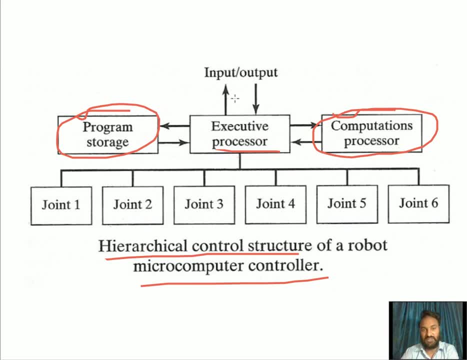 and commands are generated. okay, so input and output signals are generated and, like in previous slide I have discussed, it goes to the feedback in joints 1, 2, 3, 4 and it again comes. farewell, it means it forms, the close one is going free来. so you see, in the joints command is given like this: the 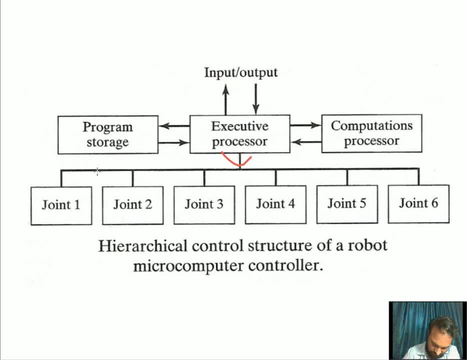 command is given like this: command is okay. the executive processor generates some signal. so signal sends the command in each joint again, but the feedback goes to the executive processor and, based on computation processor, is there. so how much we need to move again the joint so that we can reach the desired position. that's why 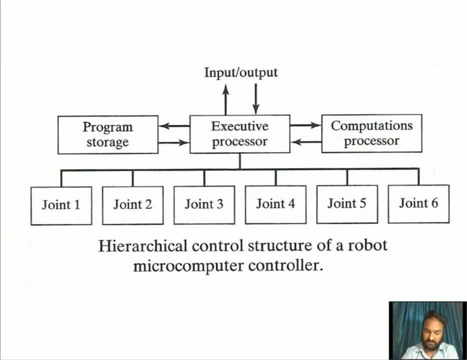 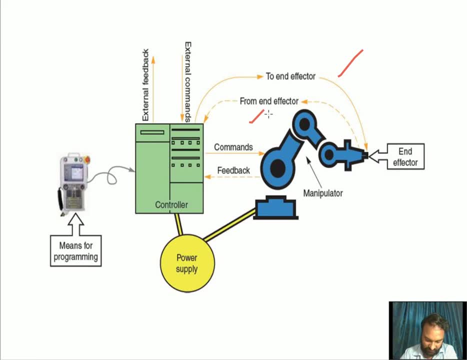 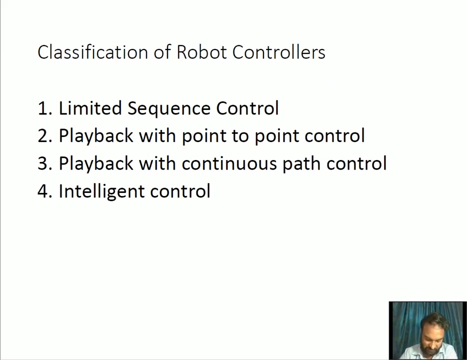 okay, next- see this, that is what i was discussing- to the end effector. from the end effector, again, power supply, external feedback, external commands are given and this pendency is used to record the signal. okay, so classification of robot controllers is mainly classifying under four category: limited sequence robot play playback with. 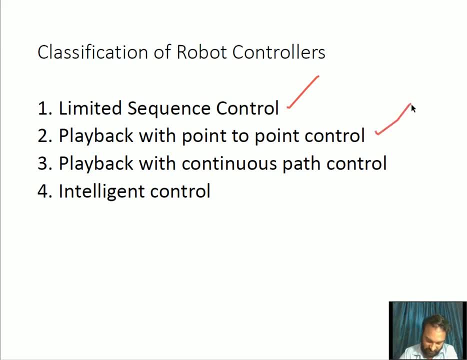 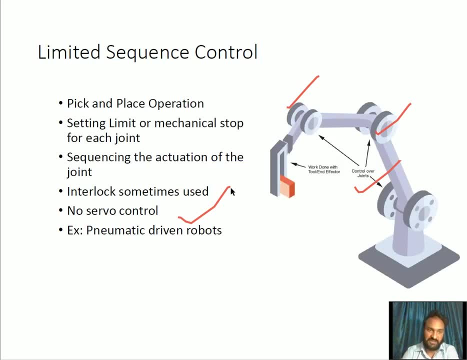 point-to-point control, third, playback with continuous path control and fourth, intelligent control. we will see one by one. so here, limited sequence control. this is particularly useful for pick and place operation. type of operation setting limits are making this stuff for each joints. so how we control the, actually we 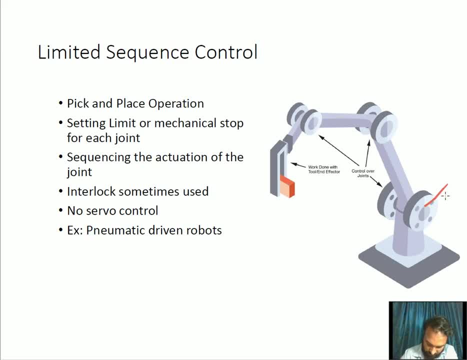 how many joints- one there can be, one here, one here, two, three, four and five, six. okay, say, five or six joints are there. so we need, for a particular location, this one. we need six value of and in the form of angular angle for all these six joints. we will see. this one is: 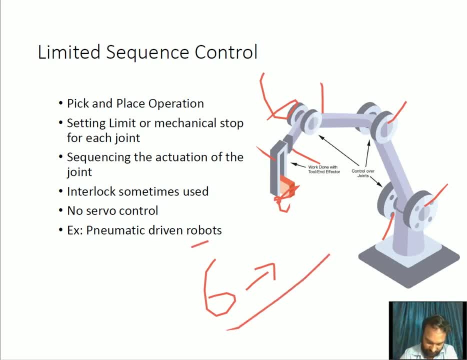 coordinate system but for, for instance, just remember that to record the location we need to generate six coordinate value, or say six angles for one, angles for each joint, and if there are six joints are there, that means we need to record six angular position, and if there are six joints are there, that means we need to record six angular position. 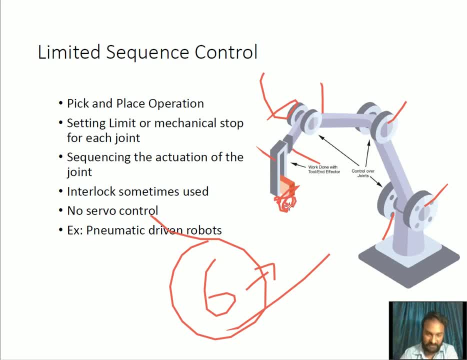 only then it is able to achieve here this place. okay, so if the point to point control, if it is moving here, then again to reach here, each joint position will have this, some different angular position, and that angular position is recorded for each joint and again it means how many angle position we. 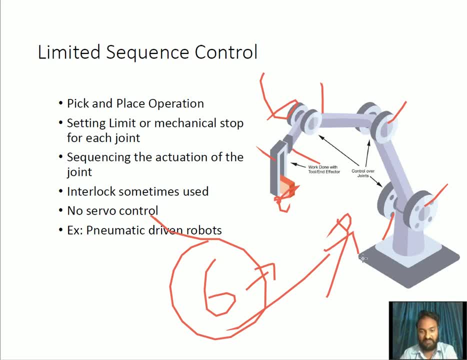 need to record. if there is five axis robot, then five in five axis, then five and six is, then we need to record six. okay, so in particular case in this one limited sequence in where we don't need various motion, so we need limited motion, so for that picking and placing type operation is enough, so here we can set limit for. 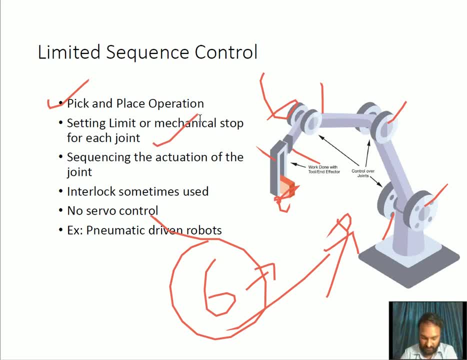 mechanical stuff for in joints. it means we can set the limit. for example, this joints will move only up to this angle. okay, that this one is maximum location, okay. and again, we can set the limit for this joint moment with the use of mechanical stop, then sequencing the actuation of the joints. so how the joints? 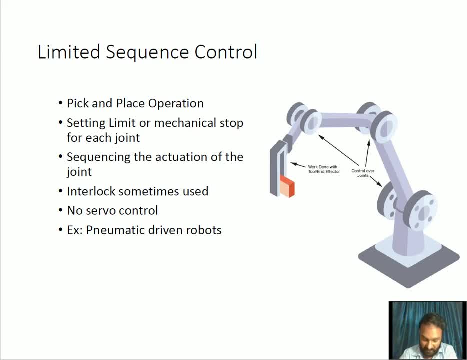 are actuated. as we record the signal during programming we record the joint location. so you location is recorded for this one, then this one, then this one. so in that way each angle of vision is signal is given for each in location of these joints. okay, first this in the position achieved, then this angle of vision is achieved, then 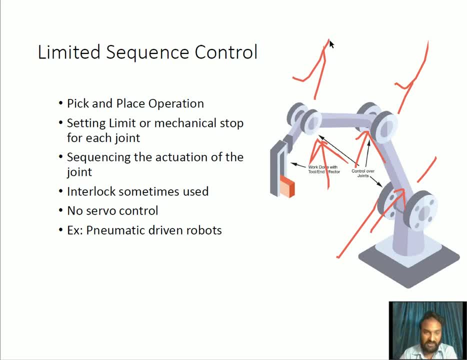 this angle of vision is achieved. so this is called. this is called sequencing. the actuation of the joints means the joints are actuated in sequence, not simultaneously. okay then interlock. sometimes with interlocks are when you limit the motion of the robotic arm. so, for example, you can use interlock and the back side of this. 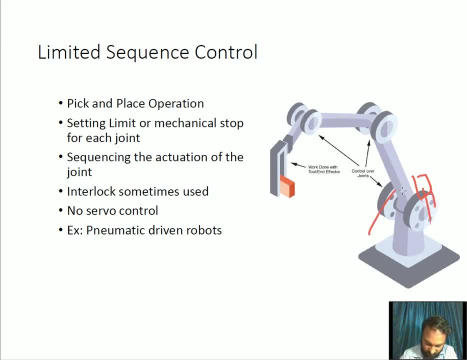 joint. okay, so you need to move with the robotic arm only up to this angle so you can use the restriction. you can restrict the joint moment here, so it is called interlock. so this joint cannot move beyond this angle. okay, there's a range. that is the妳 cần để lutzworkeryears- Irish. 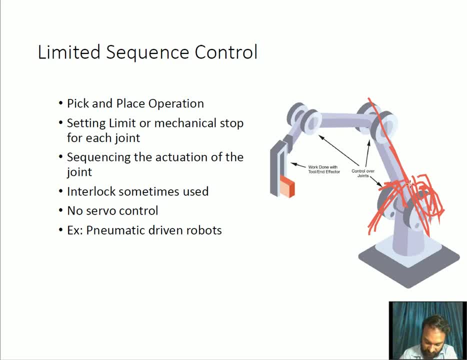 this angle position. so, once this angle position is achieved, the next joints is actuated. that's how, again, this angle position is achieved. once you, we have achieved this one, the next joint is actuated and this angle position is the one is given to achieve this angle position. 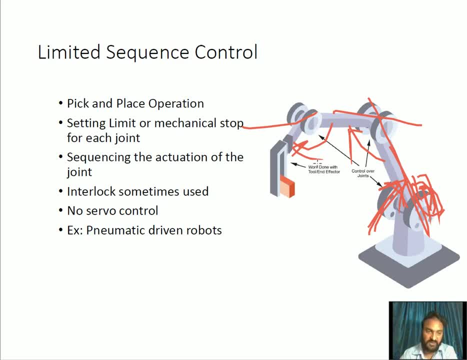 this way interlock works. again. in this no server control есть used for the point to point because this is not required, so point to point only. so no server controller is used, and generally it is used for the lighter vehicles. so pneumatic avian robots are generally used, then playback with the point-to-point control. so here 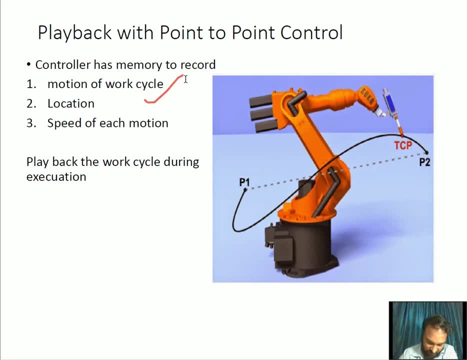 control way is very easily executed under Vietnamese lukewarm water. control may be in another two, social and others may also be available for normal light lab. then playback with point-to-point control. so here control has memory record, motion of work cycle, location, speed of each motion. so playback the work cycle. 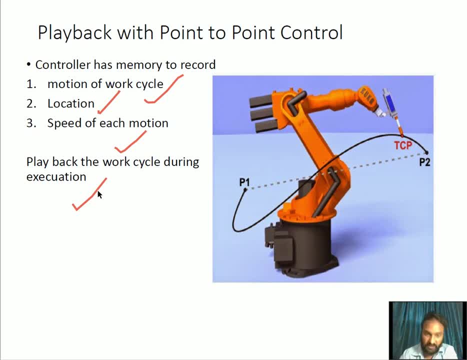 during the execution, so during the teaching here, teaching the robot, say point one, two, point, you have to move. point one, two, point two, point one, two, point two. then what will you do? you will teach it. okay. so the way you have to perform the work cycle, like you have a part, is there, then you have to. 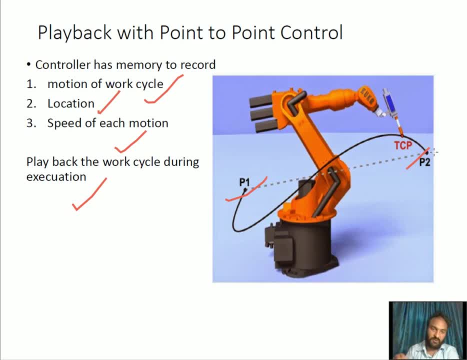 move this way. okay, so you are recording the signal and during recording the signal- this one, you see the path, this one is black- is you know the path from moving point one to point two? so actually this, all the part points on this path, generates signal. so, like i discussed, that signals are generated, what do we? 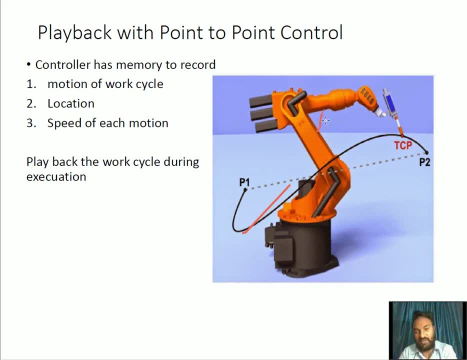 actually, how do we record the position? we record the angular position of the joints. so each path, each point will generate numbers of angular position. so if this five axis robot, five angle, for each point, for each point, five angular position will be recorded. so from one one, two, point two: 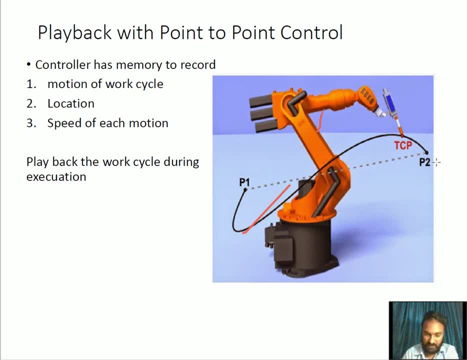 point two: there are a thousand or many numbers of points, so each, each points will have six uh, five or six, as per the robotic axis, uh value and that is recorded. and once it is recorded, during playback robotic arm perform the same way, same, follow the same path, because we have set the 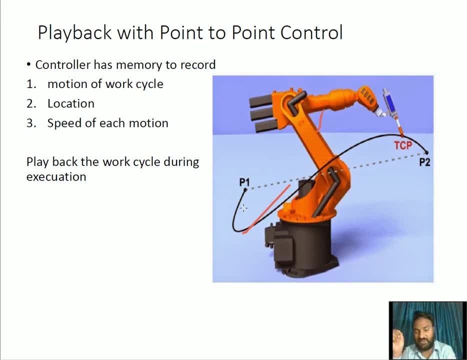 we have recorded the location and during location recording we have, we are actually recording the joint position. that's why it is able to follow the dead part. okay, so suppose point one is there. so if four point one is joint position, recorded like for, uh, axis one or joint one, you will have theta one for joint two, theta two, joint three. 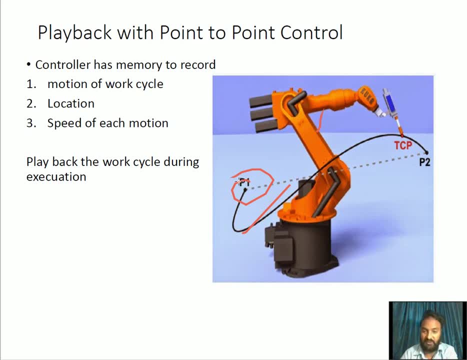 so 0.1 will have 6 value. if 6 axis robot there, the 0.1 will give 6 value, angular values. that will be recorded for 0.1 again. this one is point here. for this point again it will record 6 values for the joints the same way. so actually when robot goes here it goes this one, 0.1. 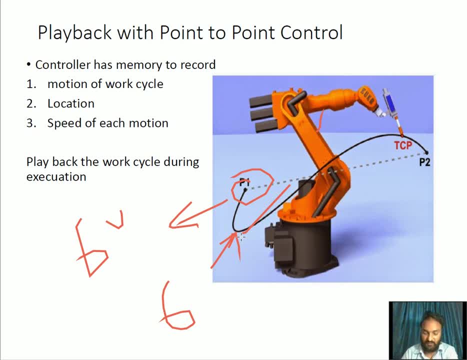 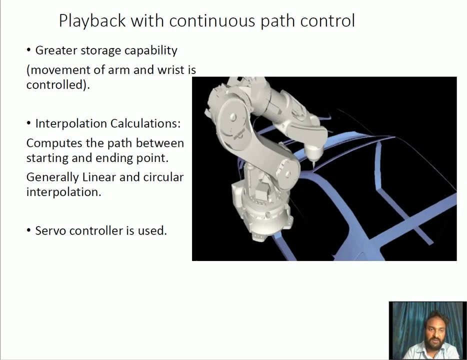 then this point: so by we are controlling the motion of the robotic arm by the angular motion of the joint. ok, that's how we are able to achieve to the point to point control. ok, i hope it is clear. then playback with continuous path control. here we need, because we are going to use continuous 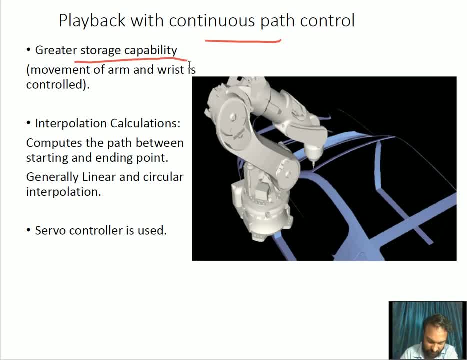 path. so we need greater storage and moment of the arm adjust is controlled here. interpolation calculation is used generally, linear and circular interpolations are used and computation of the path between starting ending point is done. ok, with linear and circular interpolation. so if you are doing the gluing operation from 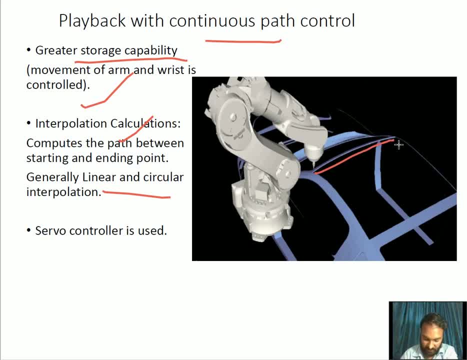 this to this way. so actually you are recording the path, so you are generating the signal for each points on this path, and since you need to generate more signal, so you need more storing capability. so again, again, we need some recording. we need to teach the robot first. only then it is able to perform. so i was discussing about teaching. 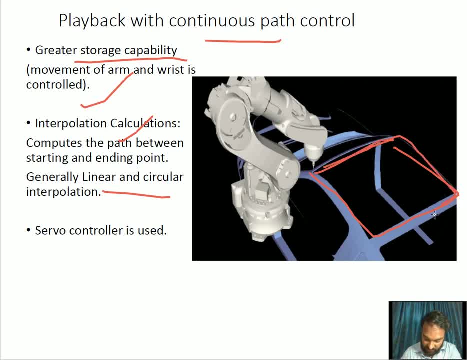 the robot, so we need to teach manually. the robot will remember the path. ok, that is called playback. so playback is like recording the path and once you have recorded the path, signals are generated, it is stored in the memory and it is going to be recorded in the memory and 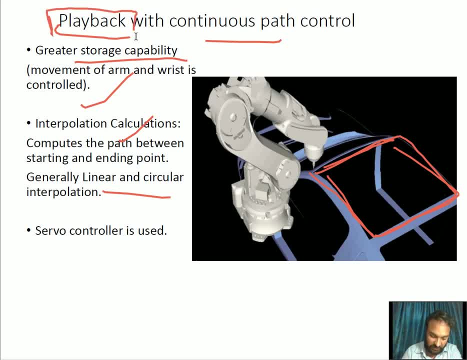 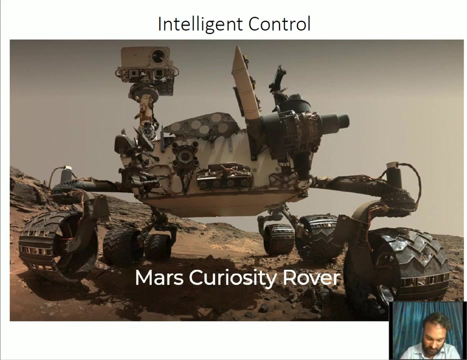 during playback, when you start the, because we have recorded the command. so when you play that command, the robotic arm follow the same path. then next is intelligent control. so this one, you see thegranite curiosity robot which is parallel drawing 01. results PDF open SET smoked update. update query: electrical server connection remote. 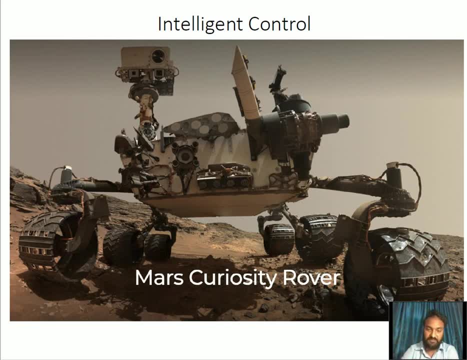 control system because, as you know, there is a severe weather condition on the Mars: very high heat and again cold, then storm, dust, storm like this, then robot, it has to cover itself sometimes. you know this need to store energy. sometimes charges better, charge its battery like this: all the commands are: 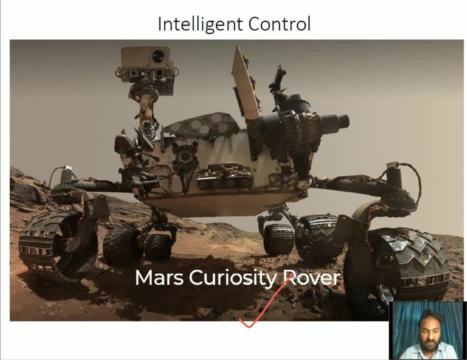 all the commands has to be have to be executed. so for that we have used the intelligence control system, like motion motion system, and different sensors are there. obviously they are able to use their own decision, they are able to take their own decision- sensors. so obviously some logical programming should be there, so so that 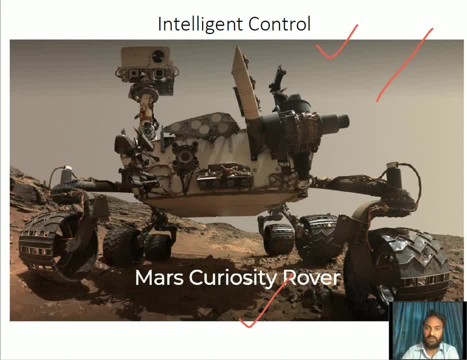 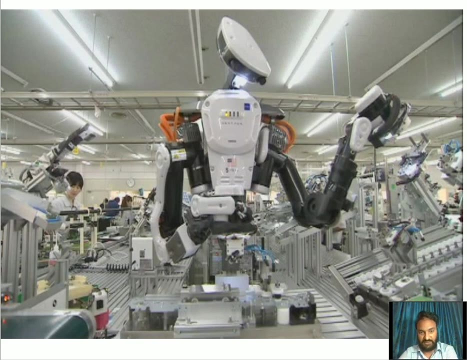 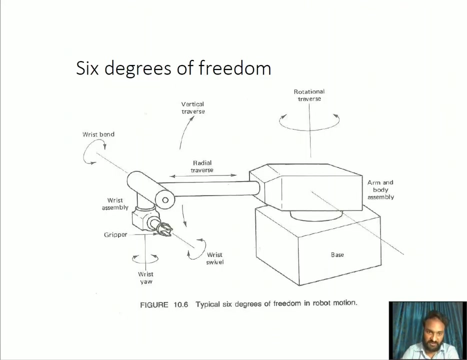 they can take their own decision. okay, so this one is very advanced system. now, this one in the manufacturing plant, if it is intelligence system, it is able to distinguish on the different part color and, based on the changing environment, it can adopt. okay, then, six degree of freedoms, as we have. 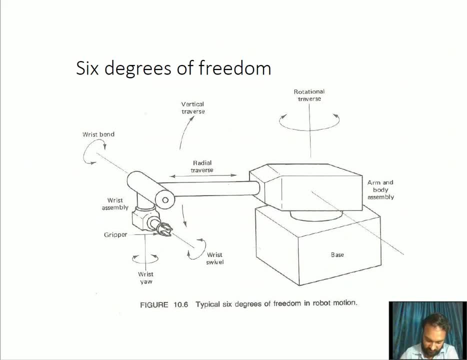 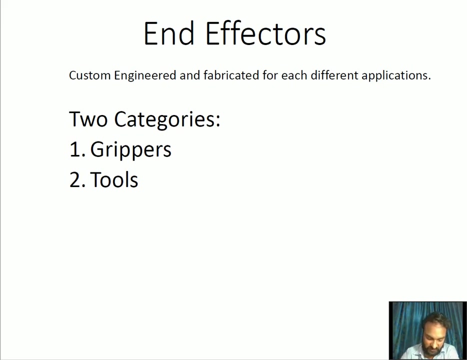 this six degree of freedom. first one is rotational showers. this one, real towers, world seed and out tower towers. this one wrist band, then again wrist yaw, then wrist swivel. we have been discussed under wrist configuration, pinch, roll and yaw. okay, so end effectors. as you know, it is mounted at the end of the 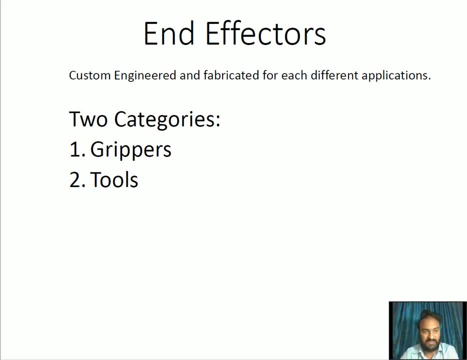 robotic arm or manipulator. so end effectors are customs engineered and fabricated for each different application as per the our requirements. we know fabricate the end effectors. so generally end effector can be categorized in two parts: grippers and tools. you will see in coming slide in two categories. 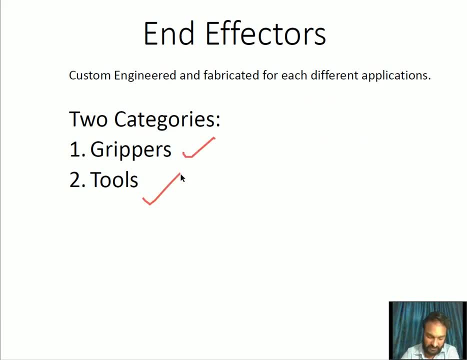 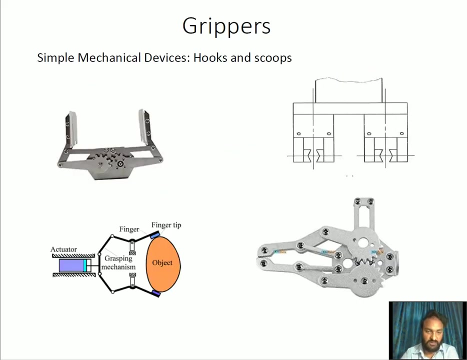 not in part. two categories: grippers and tools. grippers, where we are, we will use for the holding grasping and for the tool, we will attach some tool at the end of the manipulator or robotic arm. okay, so this. these are the example of some mechanical device hooks and scopes. these are the all grippers. it is okay. 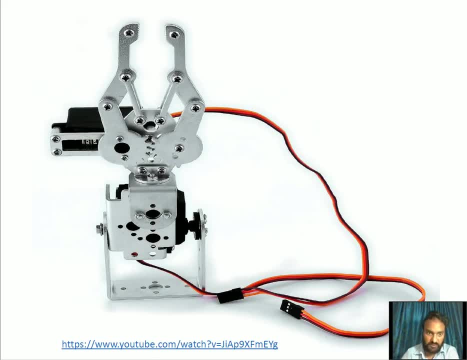 as you can see, there is not much good. all right. other one is cordless. you have otherjig machine cessation, it needs to have cordless�. all right circle. we will five jigs and then, like this, here will be alternatives for the yaw because you can see yaw drive is moving, obviously transferred and floating. 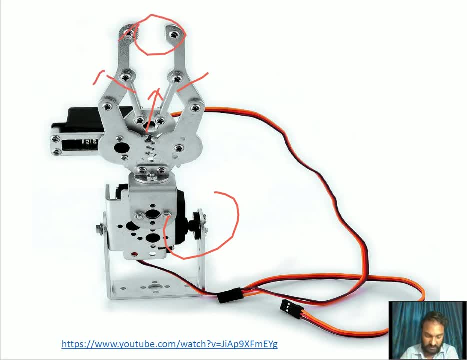 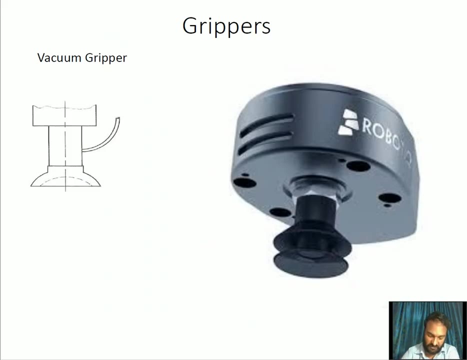 is hard, there is some function which you will need to altruize, whereas in the modern JEC is driving as you so that this jaw opens when it comes, this jaw closed down closes, okay. so again, grippers, vacuum gripper. you see, here is sucked from here, here is sucked from here when you have to open it and when 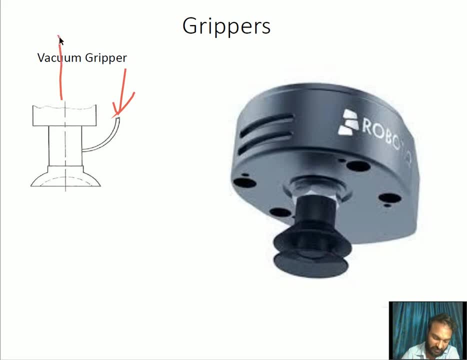 you have to open it, then you have to supply it here, and when you have to pick it, it means you have to hold the grip any part. that means then you will withdraw air from this way. when you release it, you will supply the air this way. so these are the end of the gripper. okay, what? 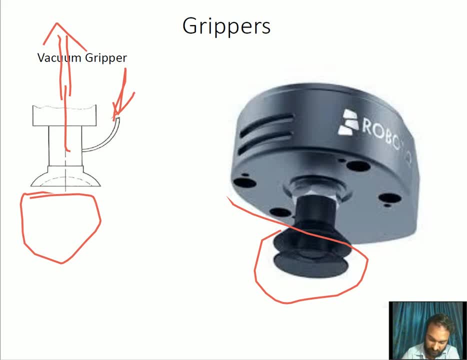 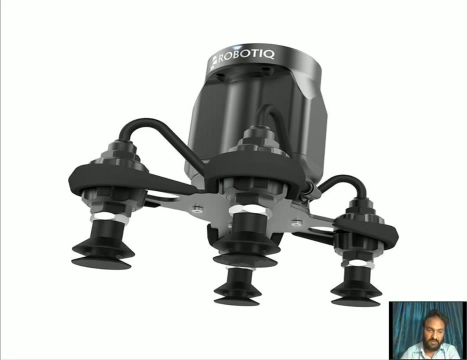 happens in this, this one. it is like a cup shape, so, like this way, when it is used on flat surface, a tight cap is made of, vacuum is generated due to vacuum generation. this one, due to vacuum generation and atmospheric pressure, is there from the outside, so part is held with the gripper, this one. another example of vacuum gripper. another example of. 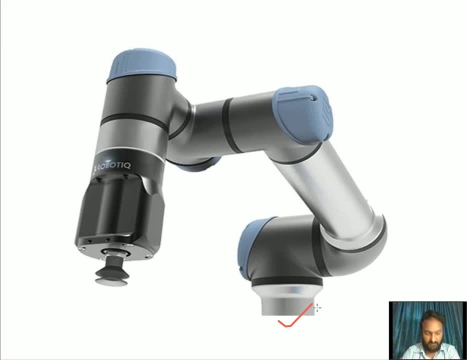 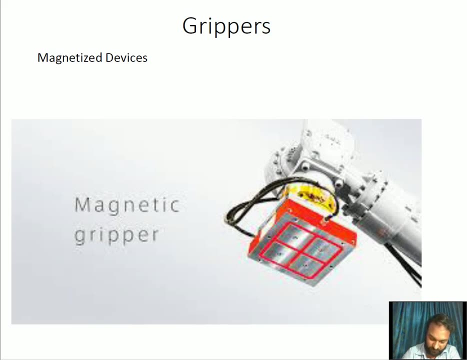 vacuum gripper. you see, then we have magnetic gripper. you see the electric surface there. then this one become. we have select LUV and that else is treated with vacuum garbage, so on. in the future I can get ¿dou surprise you. so you see, first you easiest way to clean your vacuum and部x the whole car. so next time when you prefer to start into this, 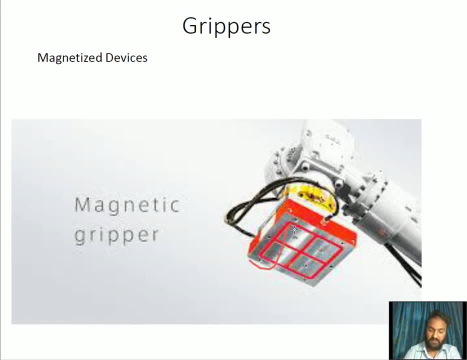 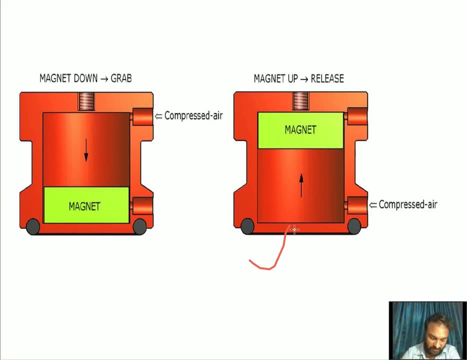 you can change the temperature to the pressure, then you also get noise. then we have guess thatorar sometime during the particular who. its mixed with water, the hilarious process. cause determine your rip, and we'll start with you. some magnetic and the ferrous alloy parts can be grabbed with this. another way here, that with the. 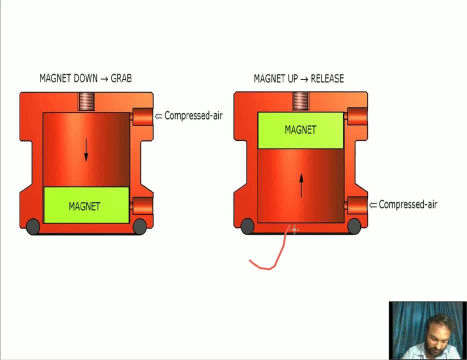 use of compressed air. magnet is there. so when you have to grab the part compressed air is supplied, magnet goes down. what happens if part is there, ferrous part, obviously magnet is there, then only ferrous part can be used. ferrous part it will come and attract with the magnet and it is remain. 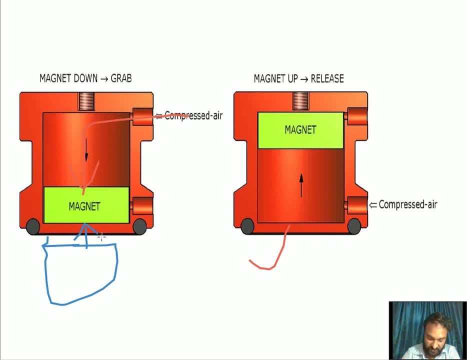 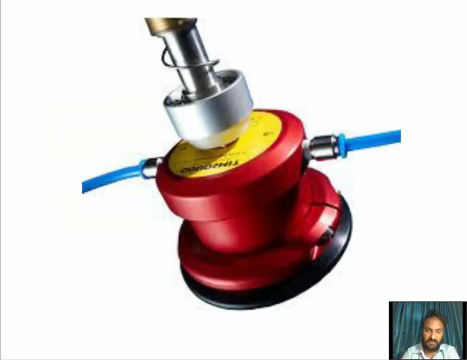 attractive, attracted, and then when you have to release it, you will supply the compressed air so that magnet goes up and part will fall, or you can simply release the part. so here, grabbing the part and releasing the part here, okay. next, another example of magnetic gripper. you see, here we generate magnet. 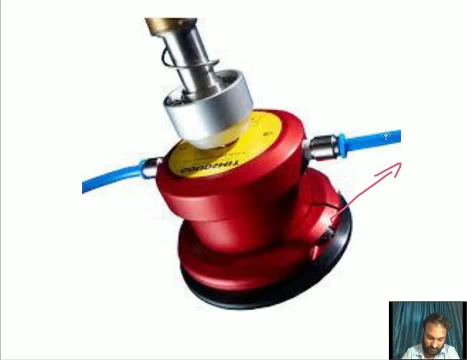 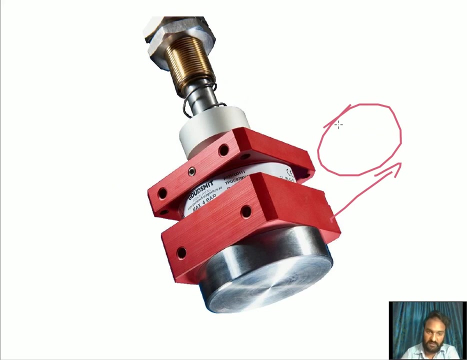 due to electrical supply. oh sorry, it is not a formula to supply, it is from where air air is supplied. so another form- you see this one here, due to it, one is utilizing the electrical. so once electric electricity supplied, this one, this one behaves like a magnet, and magnetic effect is transferred to here, this part. 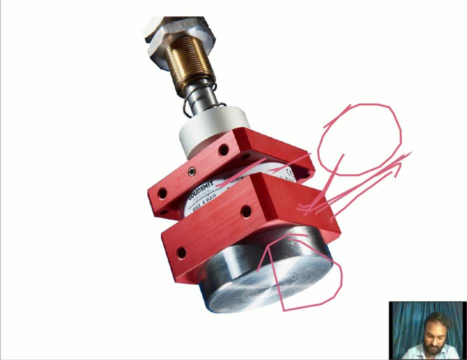 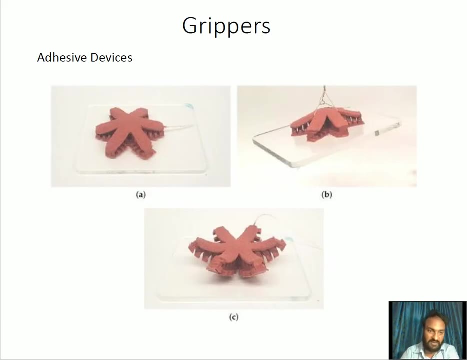 and then this one is used to grab the part. when electrical supplies card do, your magnetization effects vanishes and part is released, okay. so, like the adhesive, grip devices or gripbers are like this one. very fine structures are there and with the help of when you press it, they are able to grab the parts. 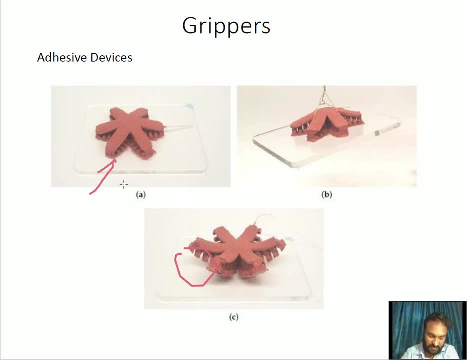 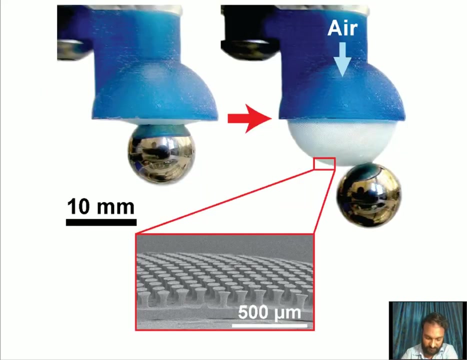 adhesive. it is not like some adhesives there, but some fibrous type are there that is used to grip the parts. so generally it generates tiny vacuum. so heavy parts cannot be handled. light parts can be handled, this one, you see. these are generating the vacuums here, in this one see. 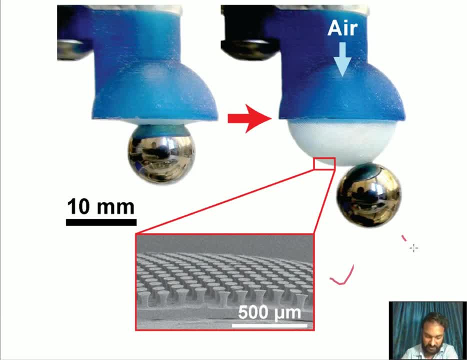 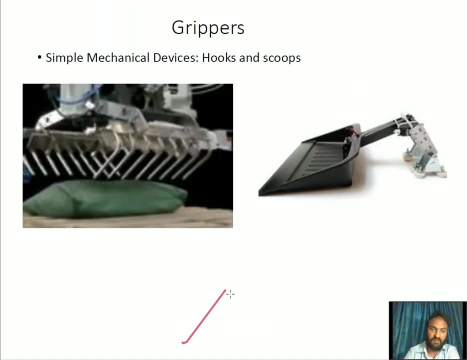 the part is scraped. here again. it is scraped here. so tiny fibers. you see here this in this one example: adhesion type paper. again, simple mechanism, hooks and scoops. this one hooksscoopsscrape that can be used for the lifting the object, generally lifting and transporting purposes. this type of leversgrippers are used. 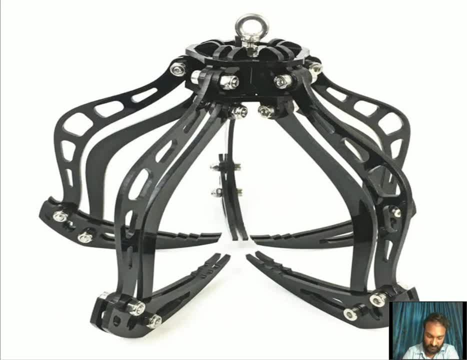 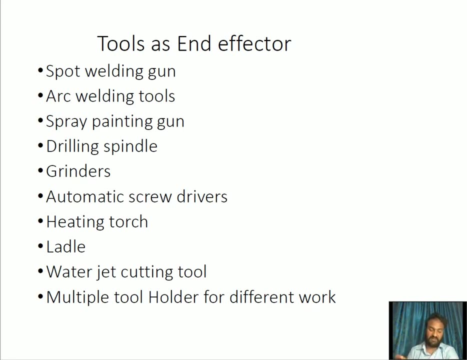 again. you see this one clog. this can be used by picking the parts, fine chicked, putting it at some particular place. so, applications of tools, tools. what are the tools? as a end effector can be used like spot welding gun, arc welding tools, spray painting, gun drilling. 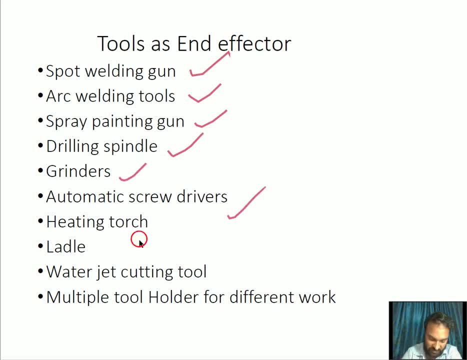 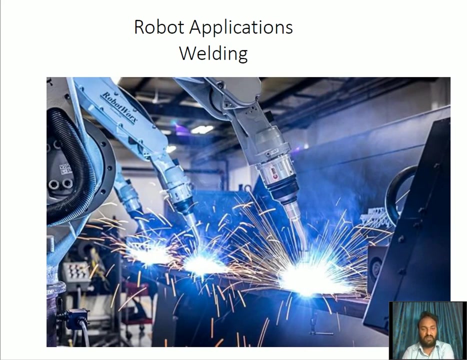 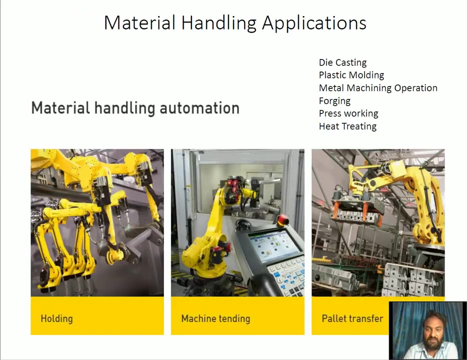 spindle grinders, automatic screwdrivers, heating torch ladder, ladder for casting water, jet cutting tools, multiple tool holder or different works. laser works can be included in this, also laser ok, this can be used as tool. these tools can be used as end effector. so robot applications includes for the welding purposes you see here. pipe is being built here then 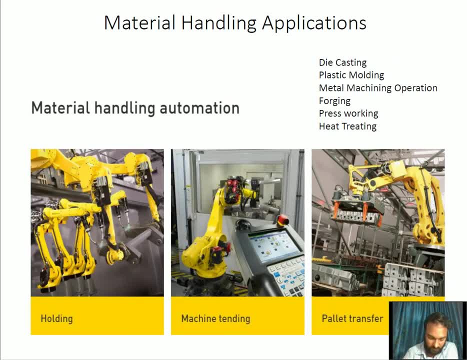 material handling purposes- material is being built here. then material handling purposes- every part holding, then machine tending, like we discussed in previous, probably in video third, that part third and machine tending, loading and unloading, along with other tasks. so part loading and unloading can be done here. then die casting, plastic, molding, metal. 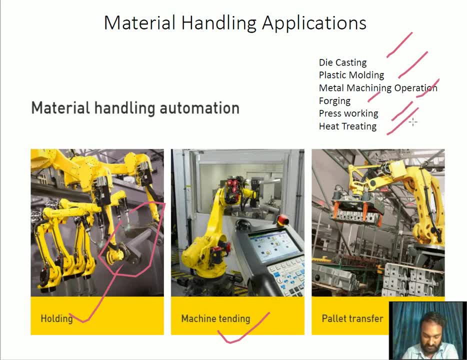 machining operation, forging place, working, heat treating, pallet transfer. here pallet can be used, can be transfered into the machine and then other equipment can be used here. this is hotvat cutting machine wasting material. this is just some of the techniques used to. you can also create your own spinning and assembly machine by using this method. we can. 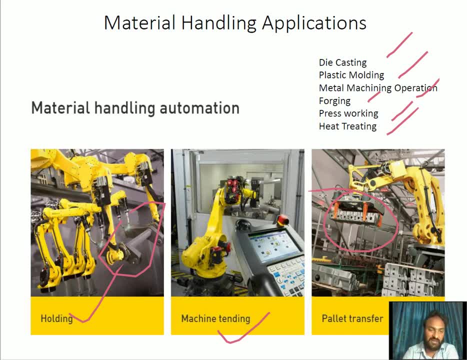 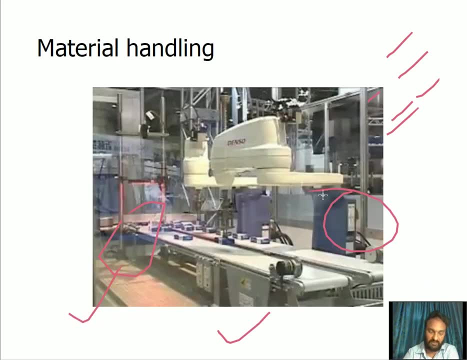 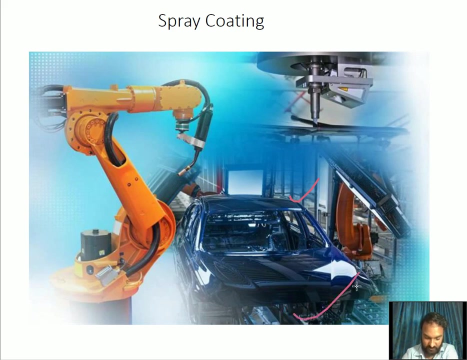 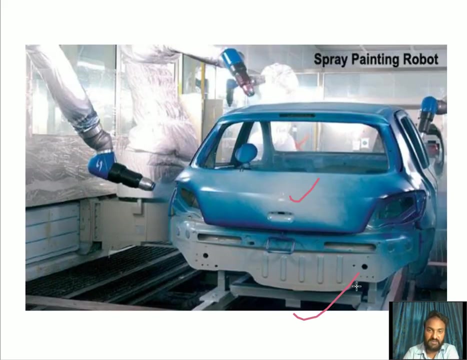 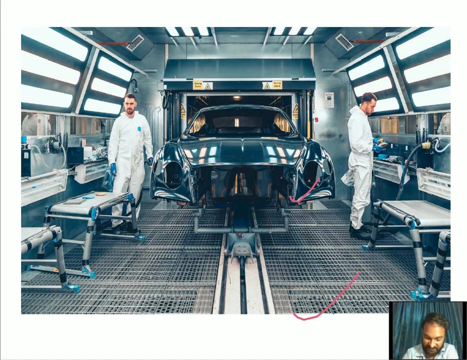 the robots. so these are all the application of metal handling under the robotic application- again this one, you see, big part is being carried away or carried by the robotic car. then spray coating: you see a beautiful car here being spray. we are spraying the paint. spray painting, again this one, such a beautiful color, isn't it? so this can be used in the spray painting. 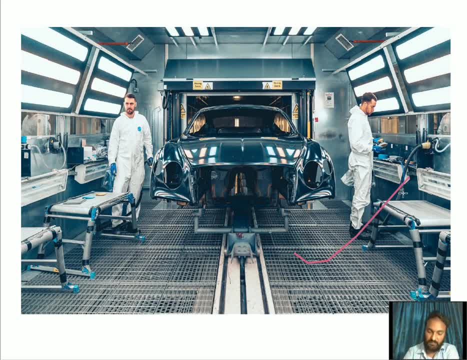 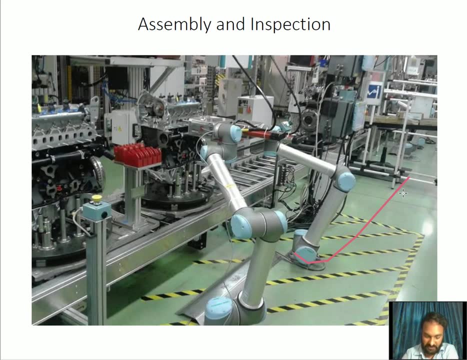 typical application of metal handling under the robotic car robot application. because, as you know, paint contains lead that is harmful to human health. that's why robots are mainly implied to paint assembly and inspection. here parts can be inspected by this one or the co-bots are there. it means these robots work with the human. 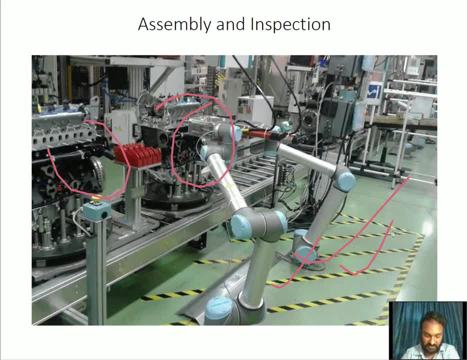 okay, so part can be inspected: dimensions, tolerance and temperature and so on. so this is the application of the robot application. okay, so this is the application of the robot application because, as you know, paint contains 2 때�ric and paint contains 2 VIS ans. all can be inspected with the help of. 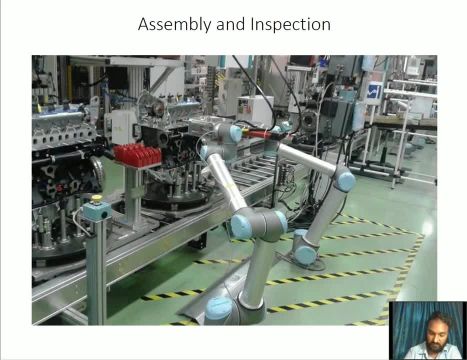 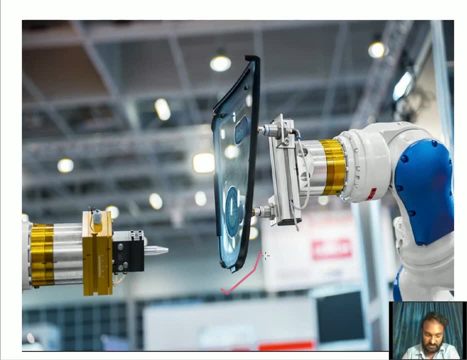 these robots. then we have material transfer. this is really began. pots can be transferred with a light adhesion grip, as you see here. adhesion gripper can we use here, not this one that is back side. okay then, now I am showing you the swatch in the plastic part of the 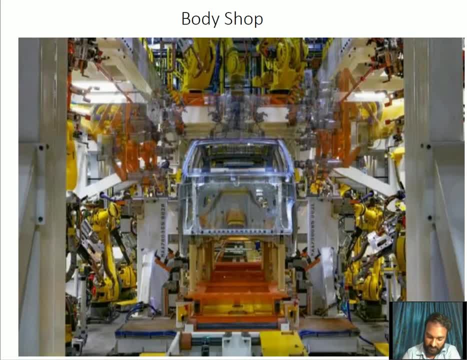 robot kit right. so basically these. you can understand that also. we just look this loading at all sometime. there is no such a lightly, but in fact we are using these gas for some things. then in body shop- see this car manufacturing company- various robotic arms are there and 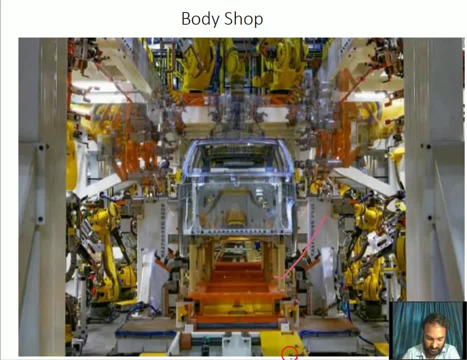 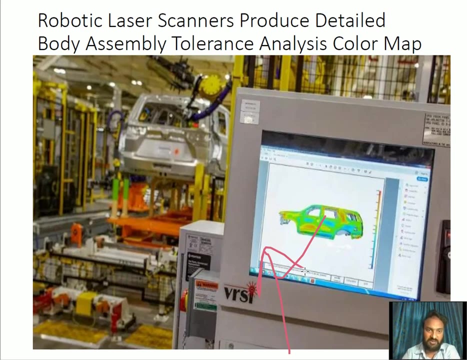 they are doing their specific task and you see, this one is transfer line. cars are moving along this line part is moving and robotic are performing their specific task. then robotic laser scanner produce detailed body assembly tolerance analysis color map. okay, body assembly tolerance analysis color map. here robotic arm scans the car and various tolerances can. 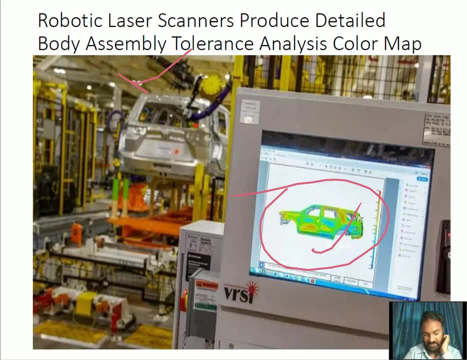 be identified. so again, this one is a typical example of machine vision system. machine vision system in machine vision system. first, what do you need? you need either scanner or high resolution camera, and then you need a processing software to process those digital images, to produce it like this, and then your display device. you can display it here like this, like computer. 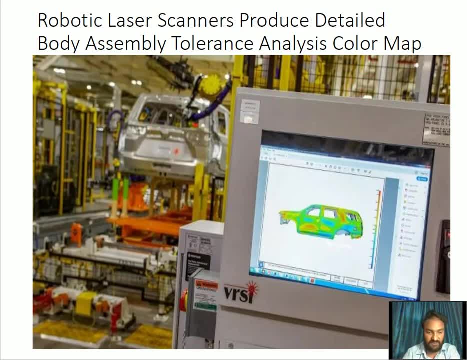 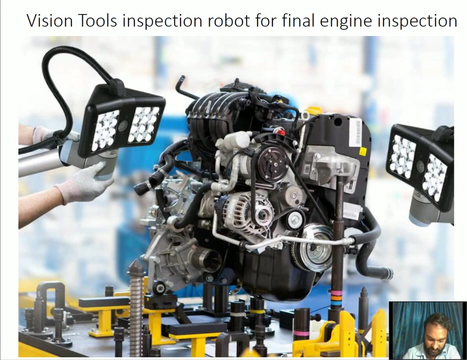 screen. okay, so these are the three parts of the machine vision system and here, without touching the parts, tolerances and stress can be analyzed using the help of machine vision system. so this one is example of robotic scanner, laser scanner, then vision tools inspection robot for final engine inspection if engine has been prepared. so